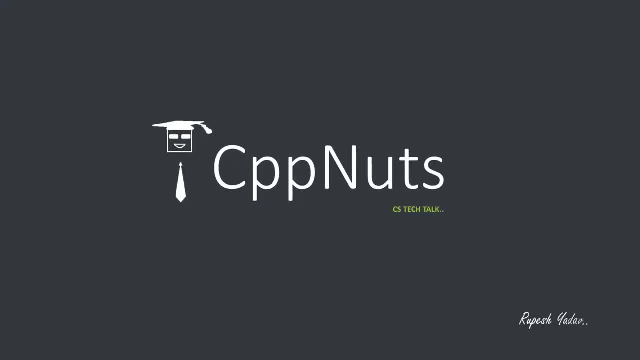 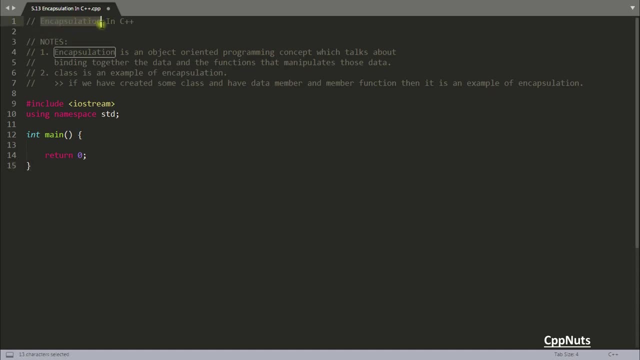 Hello friends, this is Rupesh and you are watching CppNet's video series on C++, and in this video we will be looking into this encapsulation topic in C++. This is a very easy topic and you will get it just like a snap of the finger, So let's start this. 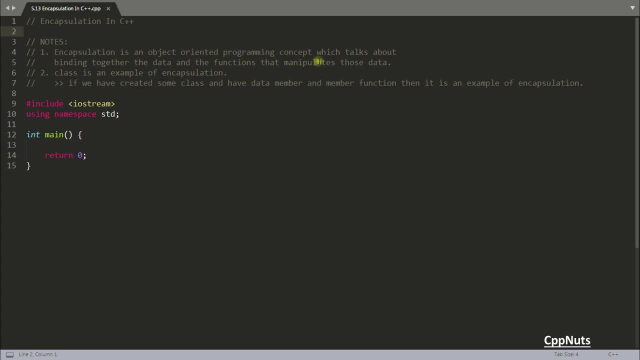 Encapsulation is an object oriented programming concept which talks about binding together the data and the function that manipulates those data. Yes, binding together data and the functions happens in class. Yeah, so let's create the class here. As usual, we will have this base class. 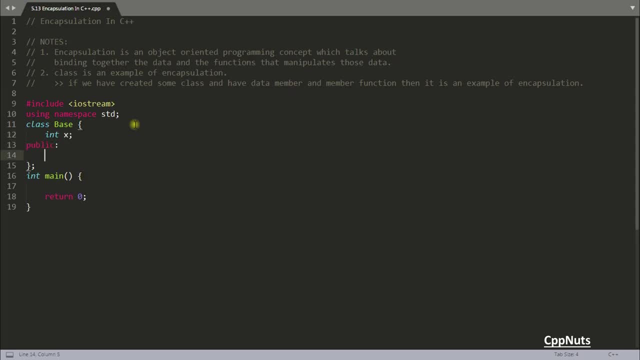 Here goes your data OK, and then public, and you will have some functions here which you will call to manipulate this particular data. Or if you are having 10 or 20 data, you will be calling those functions. So let's make some functions here. 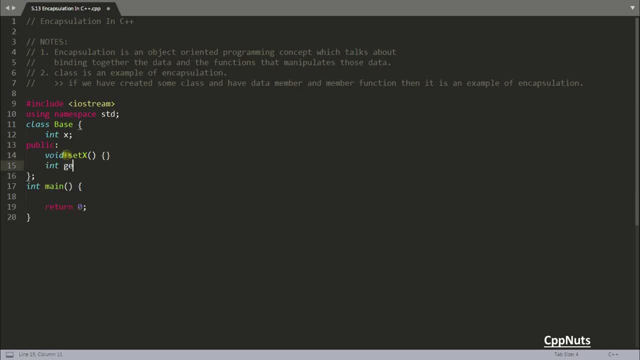 So setX, which will set the value of X, integer, GetX, which will return the X. So return X, and X is equal to A and here we are getting A. OK, so this is the function and this is the data. You encapsulated these two things in one thing, and that is called base. 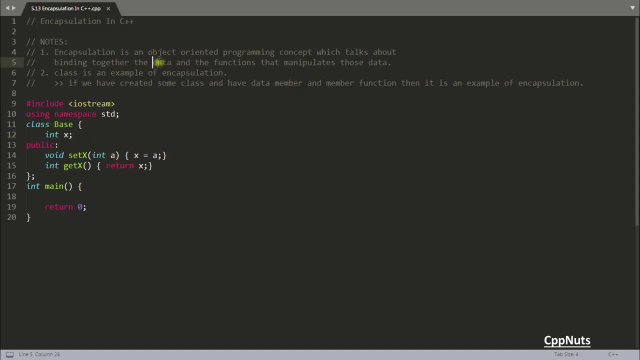 So can you see, here you are encapsulating two things: The data part and the functions which will manipulate that data. OK, so your class is a perfect example of encapsulation. OK, generally, what happens in encapsulation, Like if you are looking at some capsule that look like this: 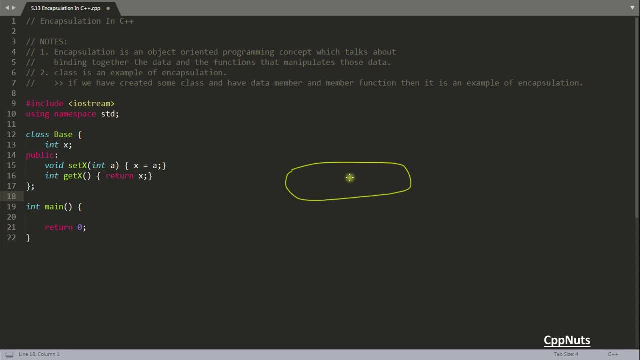 Right. So let's suppose you have some capsule. It looks like this. Then it has two part. One is a data part and another one is the function part. So data is this one, function is this one. You encapsulated these two and called it base. 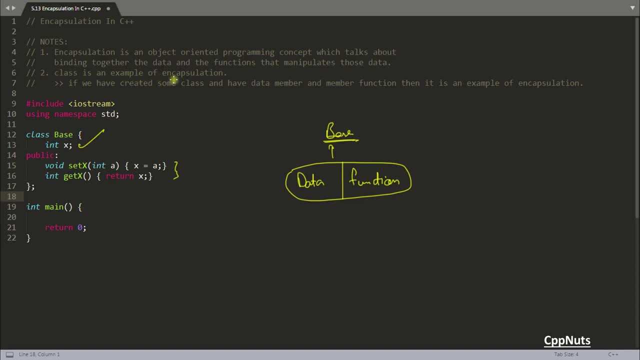 That's it. So let's read: this Class is an example of encapsulation because it does what we need And if we have created some class and have data, member and the member function, in that it's an example of encapsulation. Yeah, because sometimes what happens, you create the class, but you don't have the functions for that.